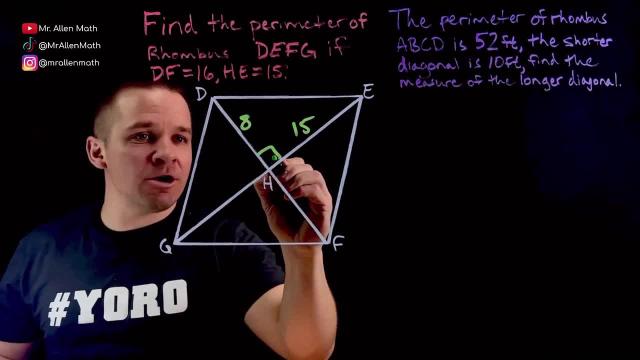 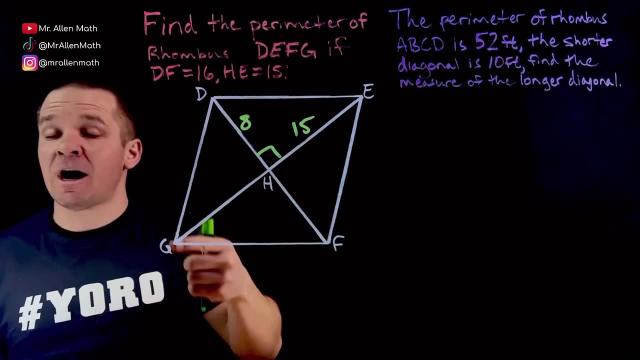 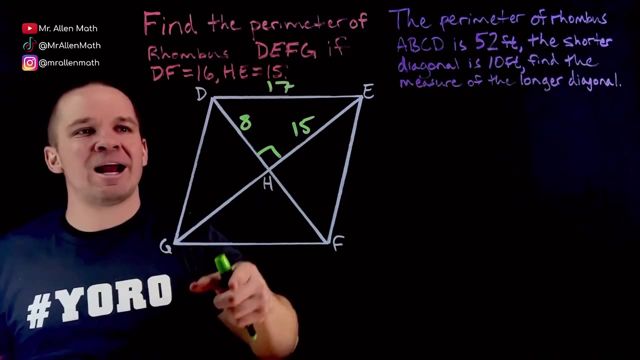 said they are perpendicular bisectors, So this guy here is a right angle. Hmm, If I want the perimeter of a rhombus, I'm going to need all of its sides. Now, all the sides are congruent, So if I find one side, I get all the sides. Well, this is an 8,, 15,, 17 Pythagorean triple right. 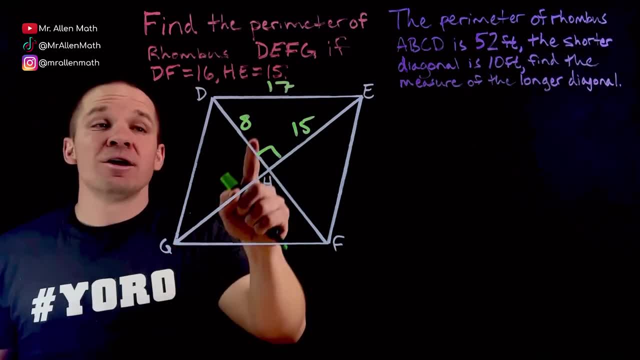 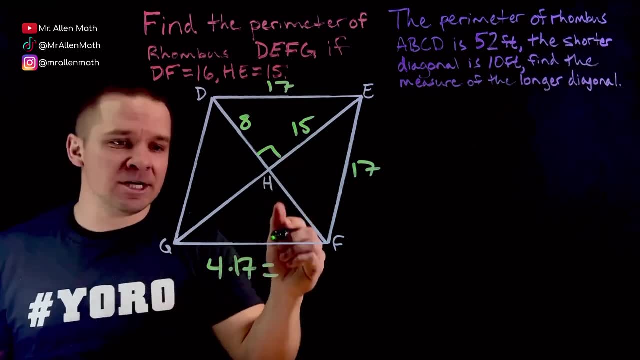 8 squared plus 15 squared equals 17 squared. So if that guy is 17,, all of them are 17.. You know, let's just do 4 times 17.. That's going to give me 34, 68.. 68.. 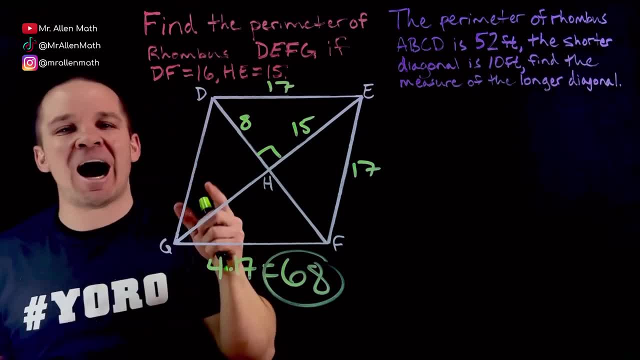 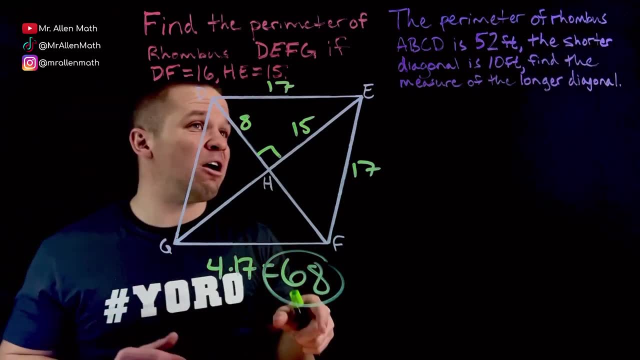 8 for my perimeter of DEFG. That's dope and awesome. We have another problem right over here, but it has, uh-oh, no diagram. Hmm, That's scary, right, Okay, Well, the perimeter of the rhombus. 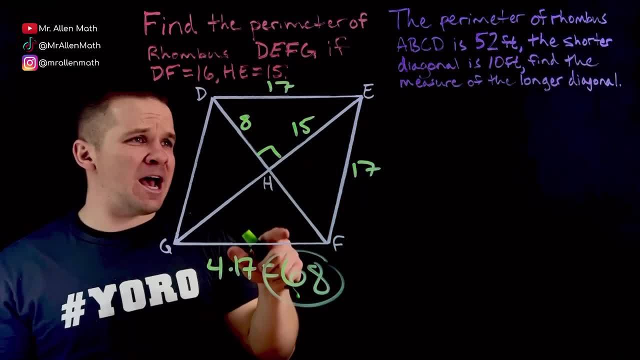 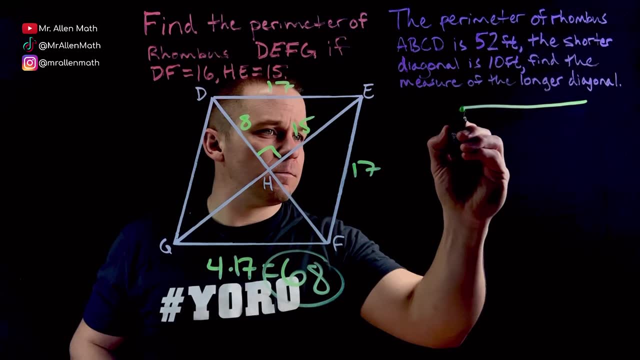 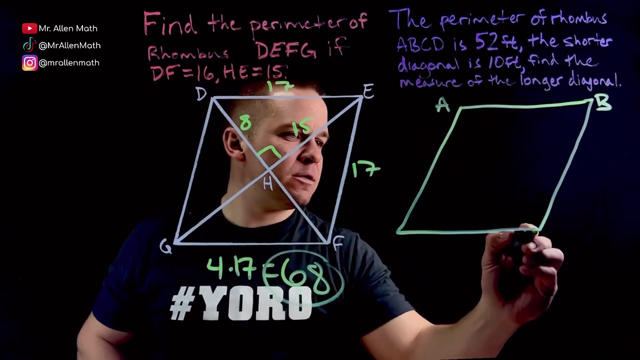 uh, ABCD is 52 feet. The shorter diagonal is 10 feet. Find the measure of the longer diagonal. So let's draw up something like similar to this one here And I'll label it AD, B, C, D. Not as pretty as this one, but it's all right, It'll get the job done. 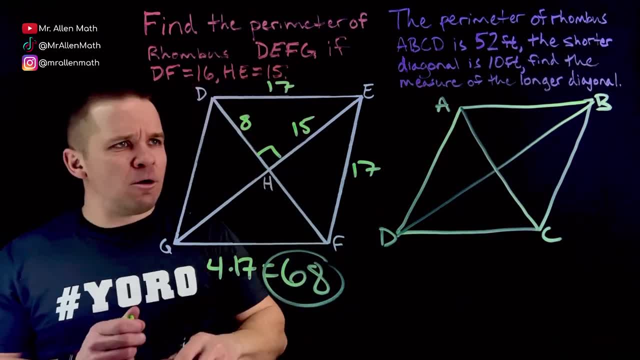 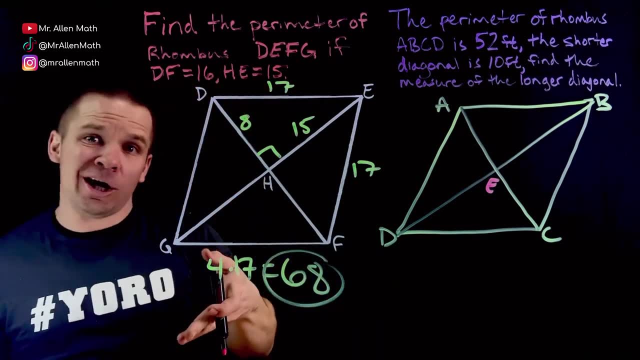 Throw my diagonal and my diagonal. Okay, So let's see, here, though, The shorter diagonal is 10.. Um, well, let's see here I'll throw like a little E action in here. right, ABCD, E is the next letter. Um, this guy right here then is 10 feet. Uh, so that'd make it this: 5. 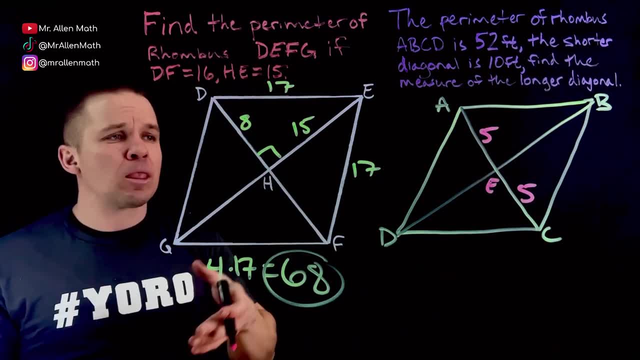 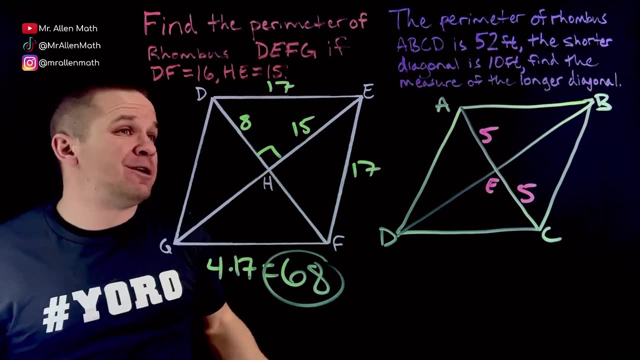 and 5, right Cause my diagonals of a rhombus perpendicularly bisect each other. They still bisect each other, just like a parallelogram. A rhombus takes all the properties of a parallelogram, which is super dope, right, But also all my. 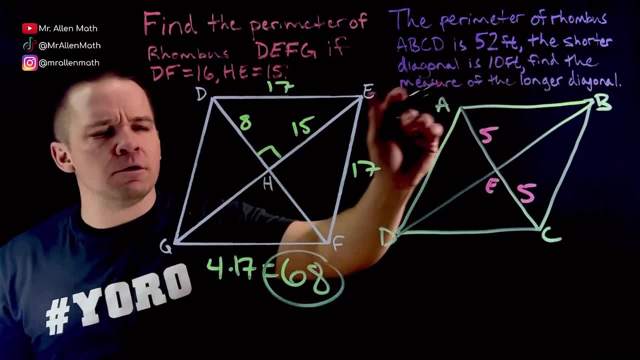 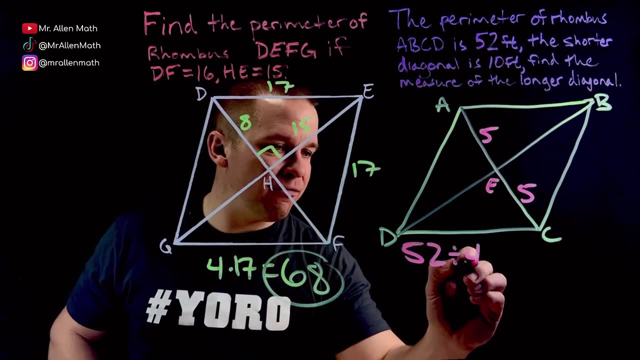 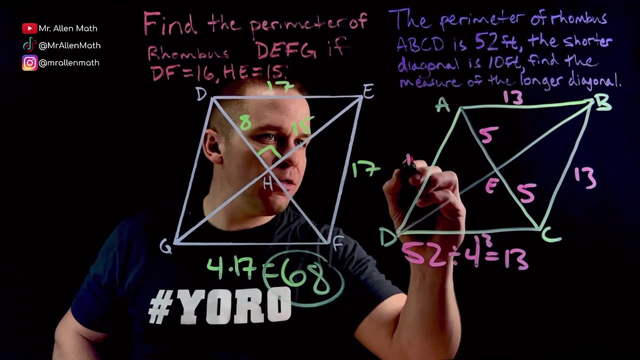 sides are congruent, which we already used here. 52. Hmm, Could I do that? But like the opposite, Oh, 52 divided by four, that's going to equal 13.. So all of these guys are 13,, 13,, 13, 13,. 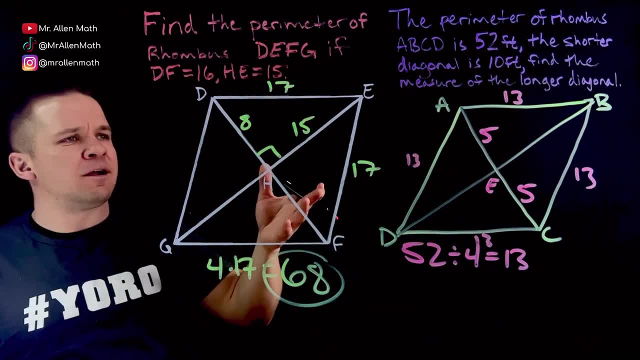